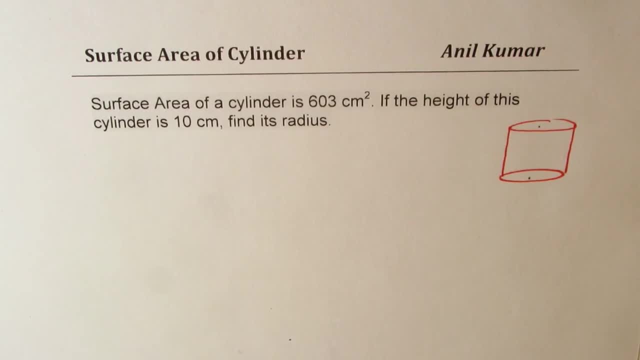 I am Anil Kumar, sharing with you an excellent question for our middle school students. It is based on surface area of a cylinder. The question here is: surface area of a cylinder is 603 cm2.. If the height of the cylinder is 10 cm, find its radius. 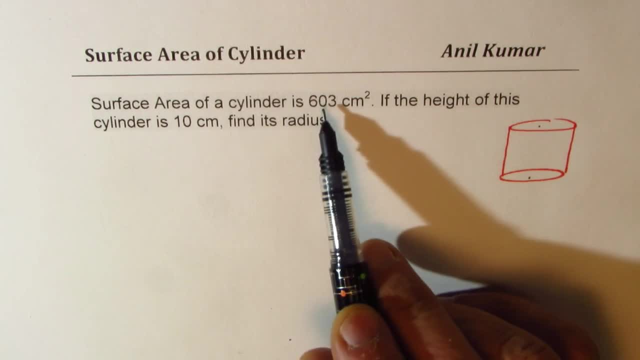 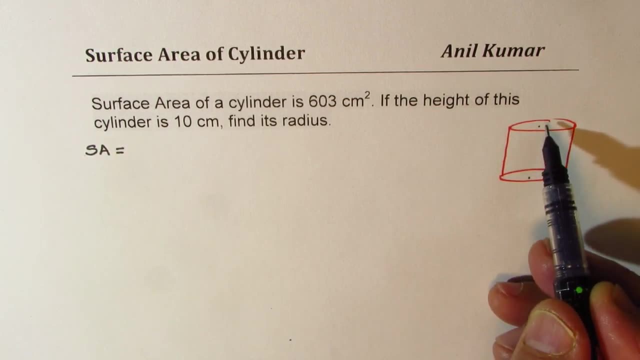 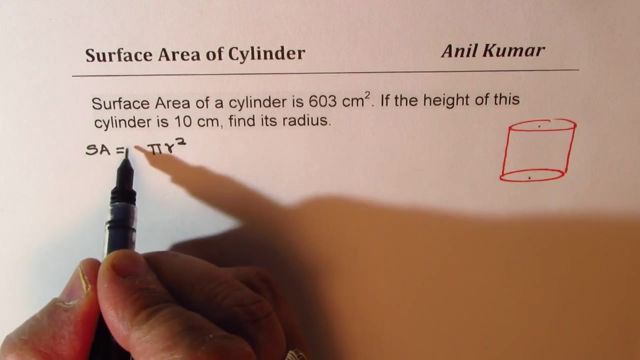 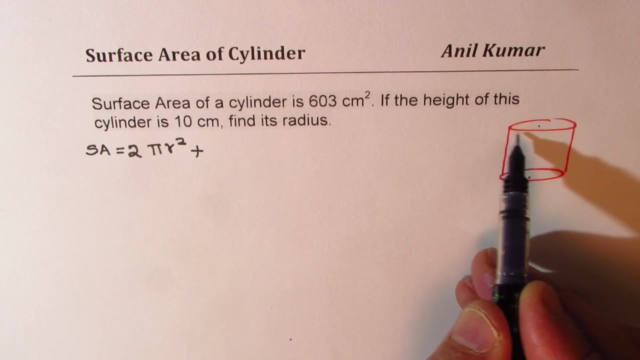 So we are given a cylinder whose surface area is 603.. Surface area of a cylinder, as you know, is area of top and bottom, which are circles right. So area of each circle is pi r square And since we have got two of them, we get 2 pi r square right Plus the lateral area of this, which is 2 pi r h. If h is my height, we are assuming r is my height. 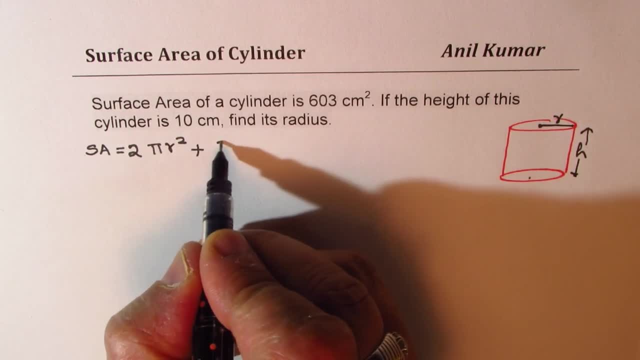 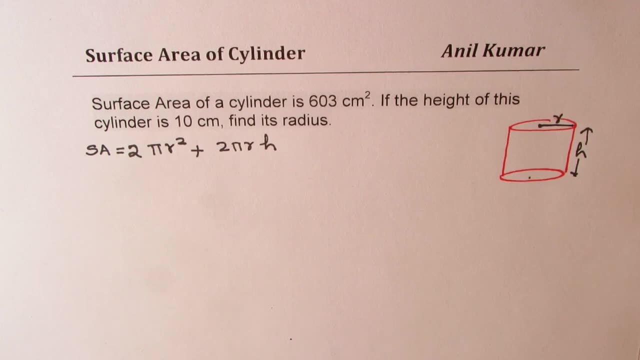 So r to be the radius of the cylinder. So it will be 2 pi r h. So that is the formula which is normally given to you and is known to you. We are given this surface area 603 cm2.. You need to find r when h equals to 10, right, So h equals to 10.. I like you to pause the video, answer this question and then look into my suggestions. 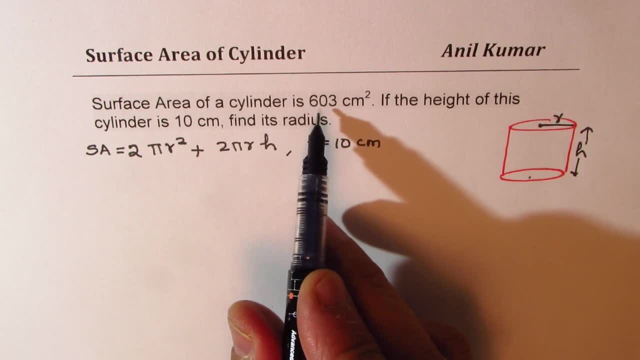 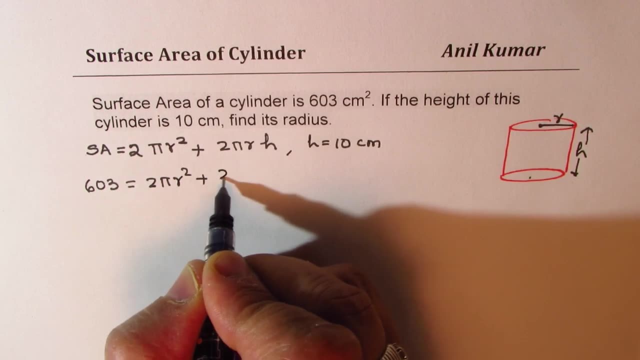 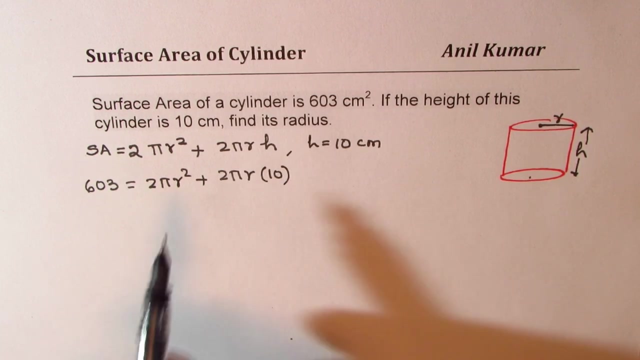 Now, if I substitute what is given to us, what do we get? We get 603, equals to 2 pi r square plus 2 pi r times h, which is 10.. So let me write 10 here. We need to solve for r. Now how can we solve? We have r square and r. That's a very difficult thing, So what can we do? 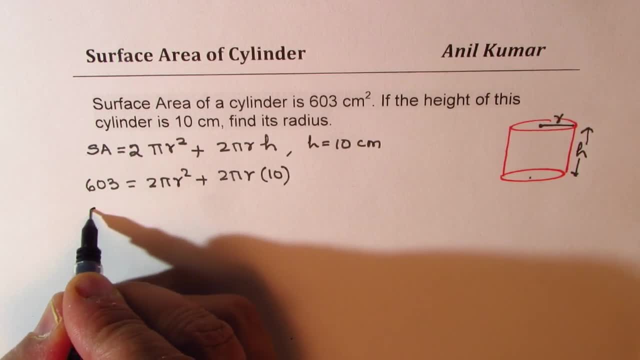 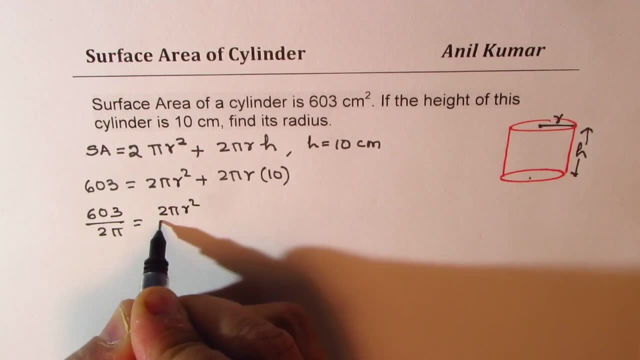 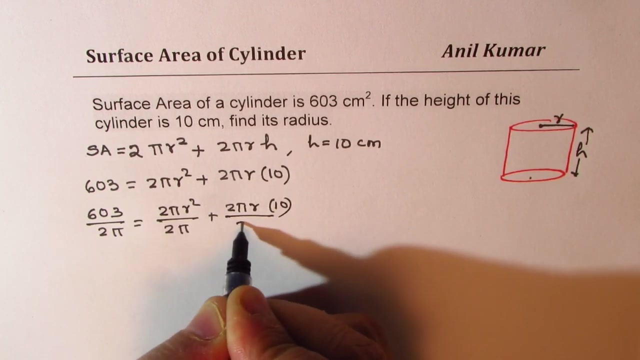 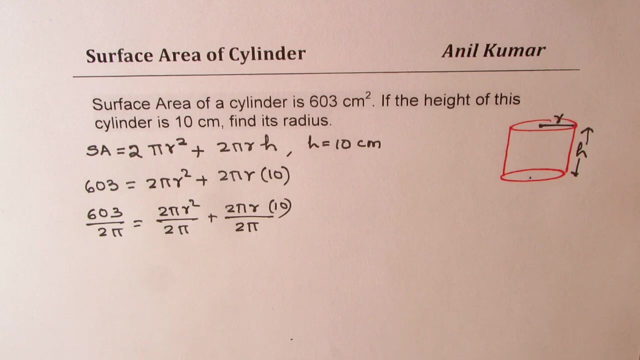 2 pi is a number. We can divide everything by 2 pi. So what do we get? Let's divide everything by 2 pi, right? So we get 2 pi r square divided by 2 pi, plus 2 pi r times 10 divided by 2 pi. So in that case 2 pi will cancel and we get a simpler expression, right? 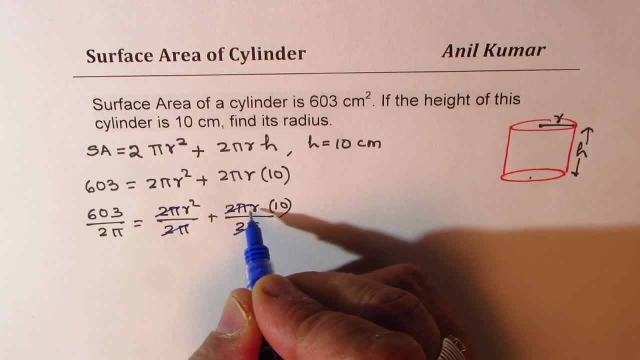 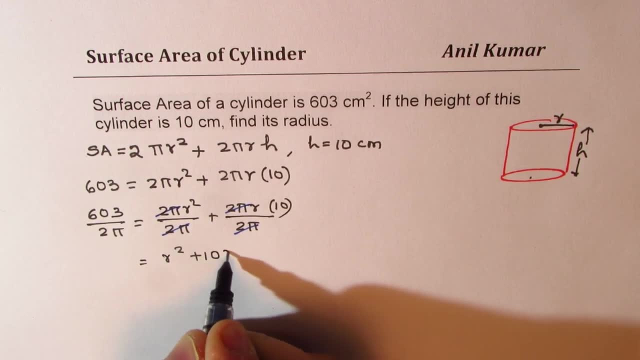 So we get this. 2 pi cancels. So we get 10 r here. So on the right side I do get r square plus 10 r. Now what is 603 divided by 2 pi? Let's use the calculator to figure this out. 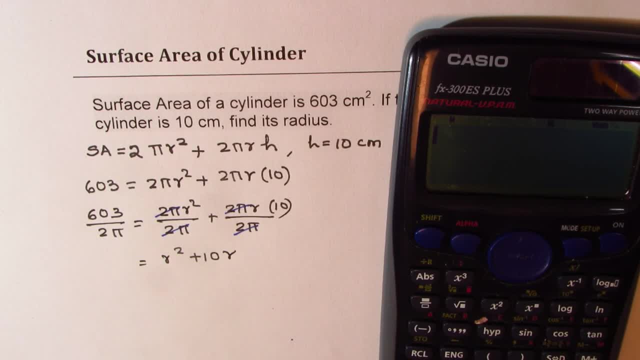 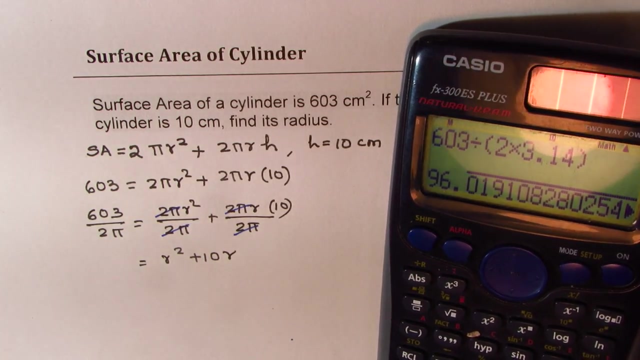 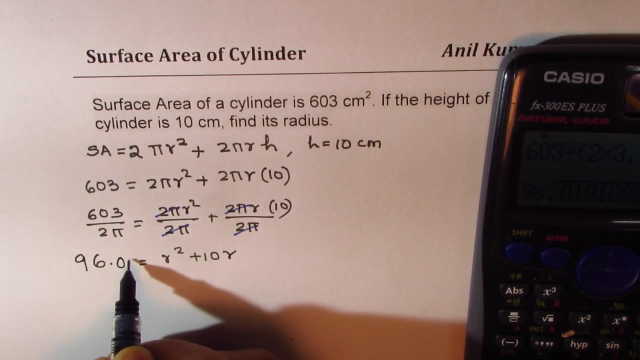 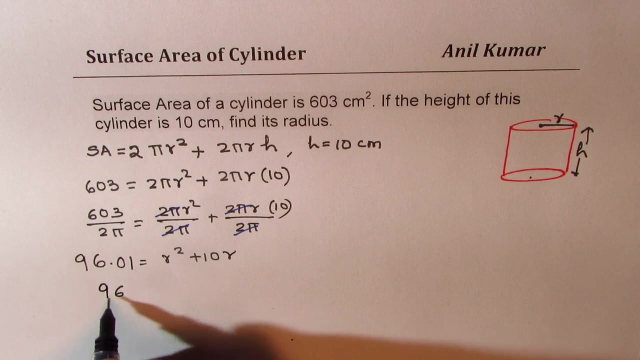 603 divided by. okay, let's do it: 603 divided by. let me write, within brackets, 2 times pi, which is 3.14,. right, So we get in decimal 96.01.. So we get this as 96.. So let me write this as 90, it is 96.01.. So let me just write this as 96.. So what we get here is 96 equals to r square plus 10 r. 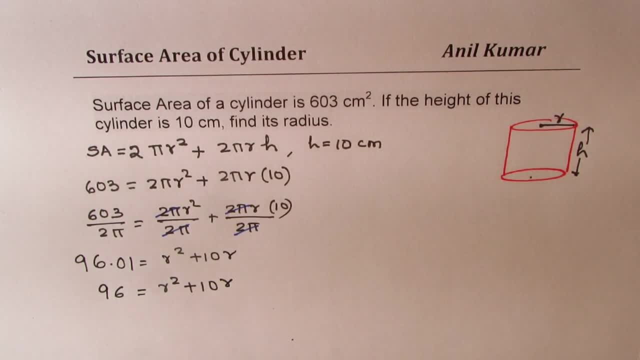 Now, how do we find the value of r from this particular equation? That is another very difficult task. Well, you can think about it and find the answer. Here is another strategy which we can apply at this stage. So what we will do here is that we'll substitute different values of r and see what do we get right. 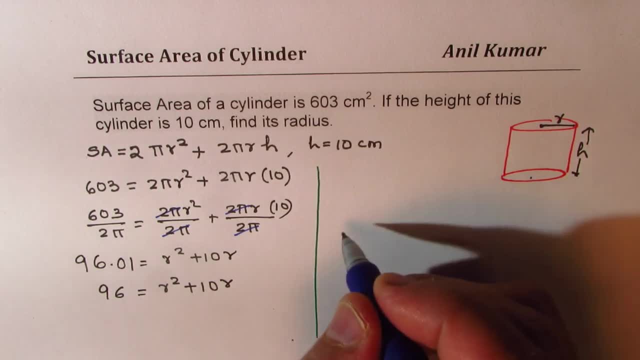 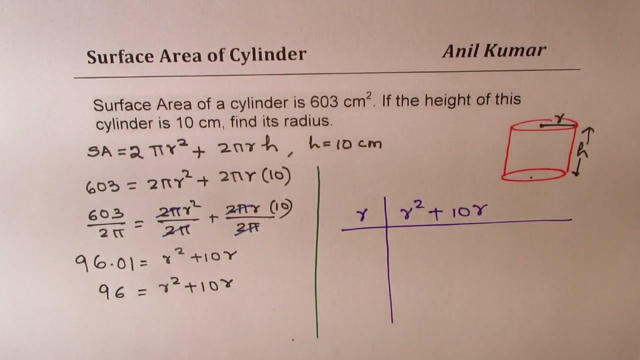 So I'll just make a table here and then substitute values for r and calculate. So let us say, if I write the value of r and then find what is r square plus 10 r For different values of r, let's see what do we get. 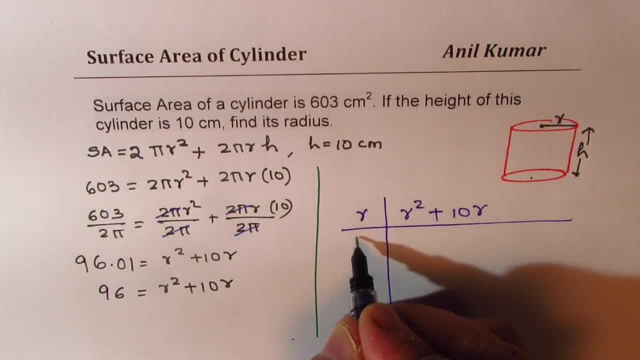 Well, let's put some value at random to start with. Let's say: r equals to 4.. Then we get 4 square plus 10 times 4, which is what 4 square is 16.. You can use calculator, right. 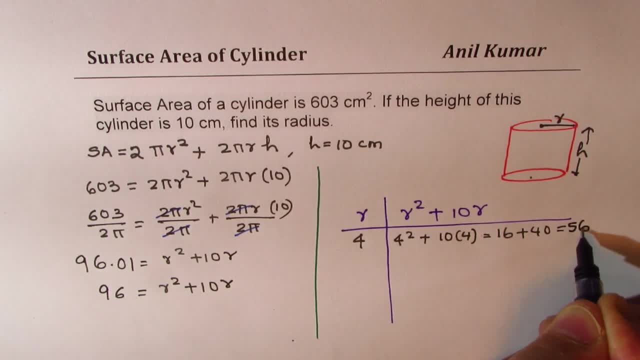 16 plus 40,, that gives you 56.. What are we looking for? We are looking for 96, right? We are looking for 96.. So that is the strategy, Correct. So you can continue with this approach. 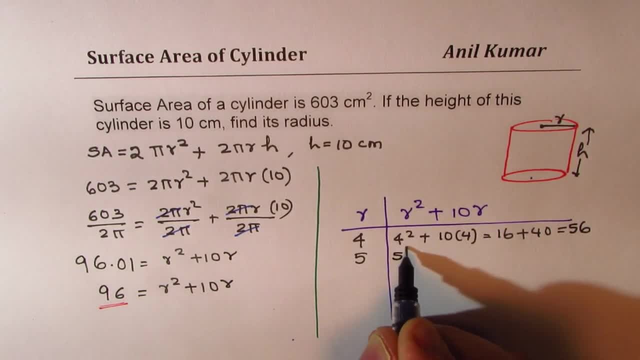 That helps. If I use 5,, I get 5 square plus 10 times 5,, which is 25 plus 50. And that is 75. We are closer to 96.. If I take 6, I get 6 square plus 10 times 6,, which is 36 plus 60.. 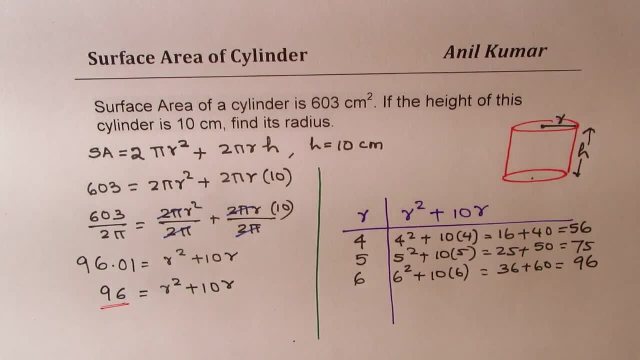 And that gives you 96.. Do you see that? Okay, So we finally get 96, for r equals to 6.. So making a table like this helps us to solve such questions, So we can write down our answer. 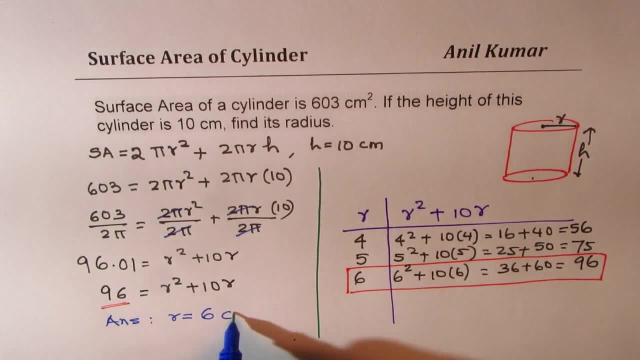 And that is r is equal to 6 centimeters. Perfect, So that is how you can find radius from the given surface area by working backwards, right? So we just substitute. We just substitute different values of r to estimate the answer. 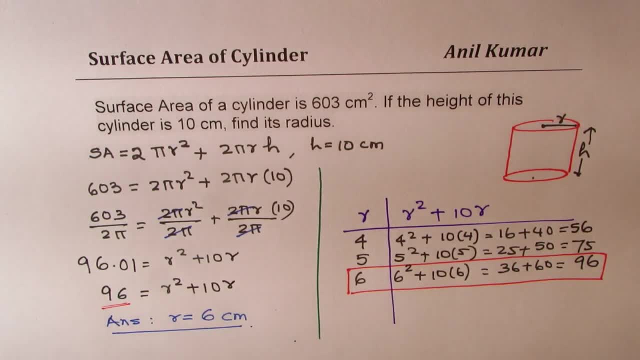 And we got exact value- almost 6,, which gave us the answer of this particular question. So I hope this strategy really helps you to think and see how we can solve such questions. I hope you appreciate it. Feel free to write your comments, share your views. 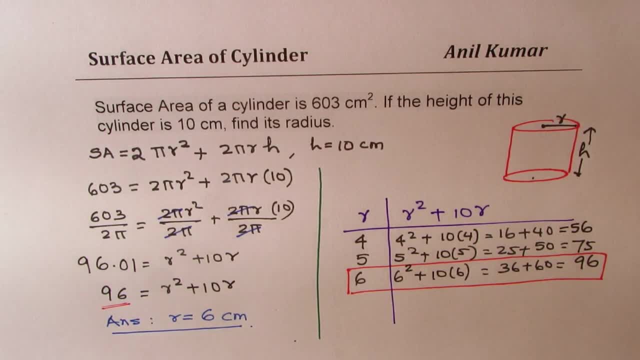 And, if you like and subscribe to my videos, that would be great. Thanks for watching and all the best. 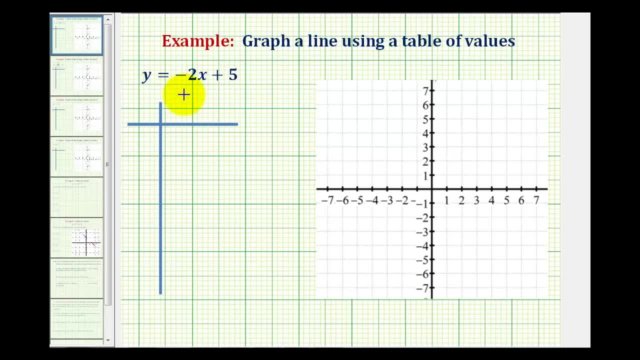 We want to graph the following line using a table of values. So let the first column represent the x value And let the second column represent the y value. So what we're going to do is select an x value, substitute it into the equation to: 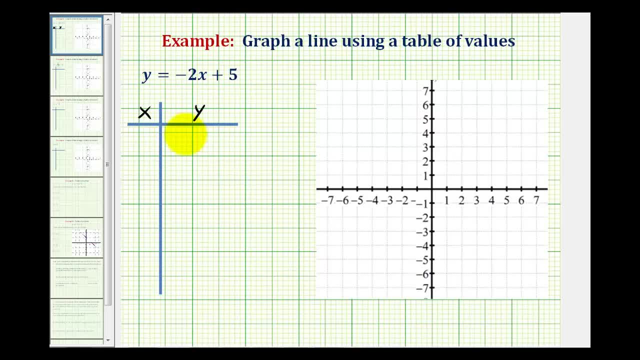 determine the corresponding y value, And every x and y value that would satisfy this equation would be a point on the line which we can plot on the coordinate plane, So we can select any x value that we want. Let's go ahead and select negative two, negative one. 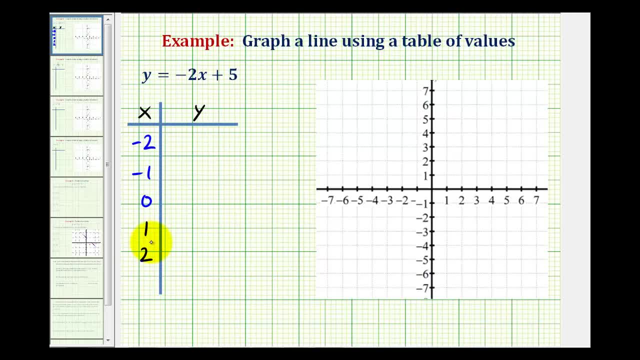 zero, one and two. Now, it does only take two points to graph a line, but we should always find at least three points. That way, if the three points don't form a line, we know we've made an error. So for each of these x values we'll perform substitution for x.